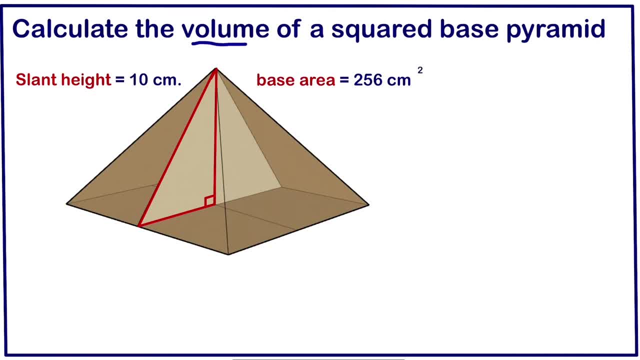 So we are asked to calculate the volume. It's always preferable to start by writing the formula of volume. So volume equals 1 third the base area times the height. So this implies they gave us the base area has been given, but we don't have the height. 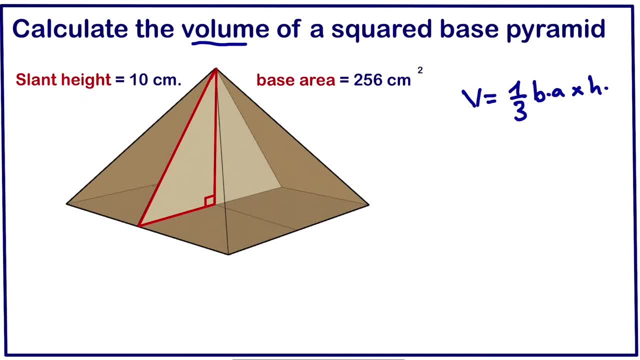 They gave us the slant height. So let us calculate the height. So, in order to calculate the height, they give us the slant height, which is 10cm. Then they give us the base area. So they gave us the base area of the square is 256.. 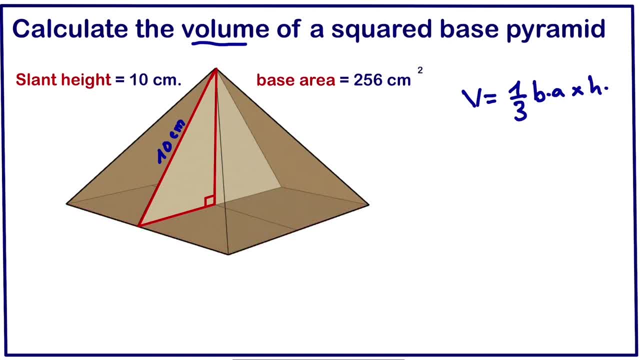 So this is 256.. So this means if you have a square, Okay, and an area of 256, this implies this is 16 times 16. so this implies this dimension is 16 and here we also have 16. so if this is 16, half of it, half of 16. 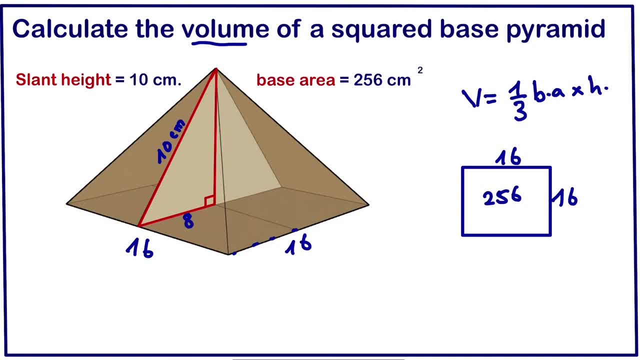 is 8, so it means here we have 8. so the next thing to do now is to calculate the height so we can apply Pythagoras theorem. so this implies H will be equals to the square root of 10 square minus 8 square. so this will give us we: 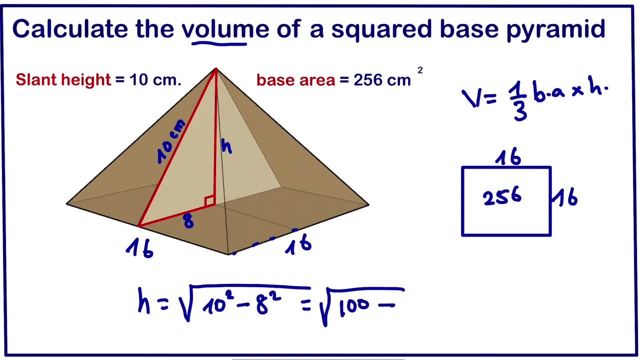 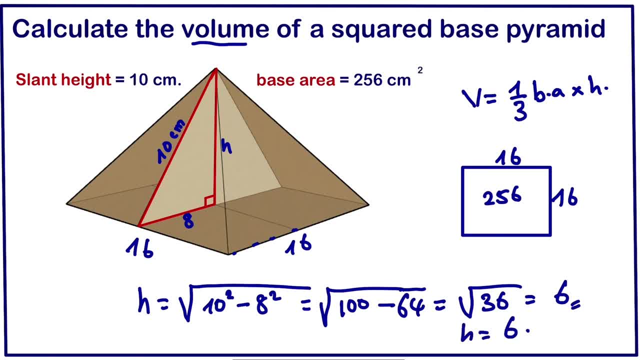 so this implies the height is 6. now that the height is 6, we can now calculate the, the volume of our pyramid. so the volume is 1. 3rd base area: the base area is 256 times the height is 6. so we can simplify: 6 divided by 3 is 2, so will be left with.